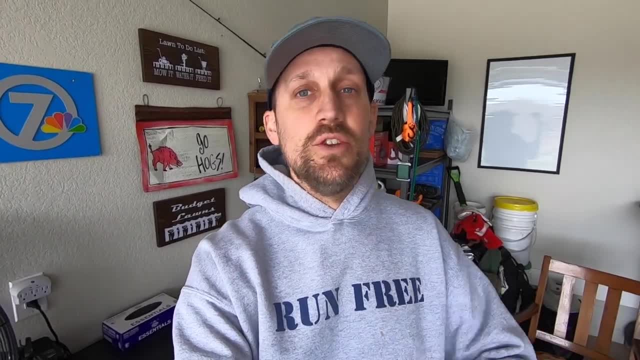 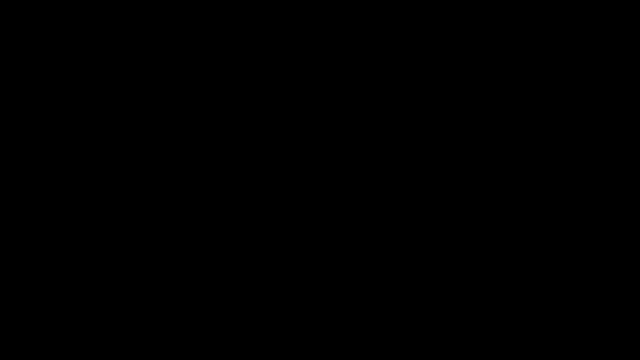 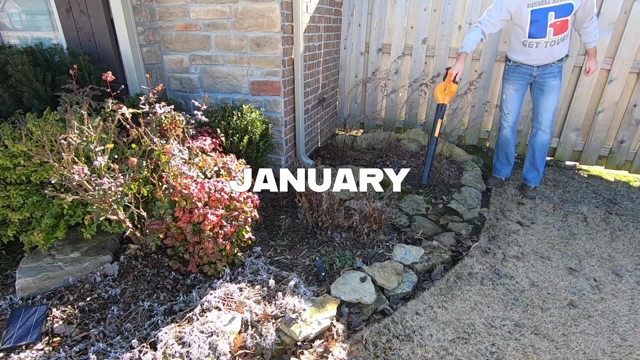 If you're looking for a video that shows you everything you need to do to your Bermuda lawn each year, all in one place. congratulations, you found it. We begin in January Now. we're not going to move mountains to start the year, but we're going to get a little bit of work done. The grass. 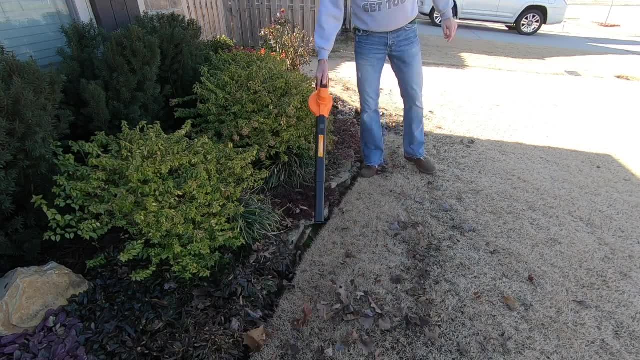 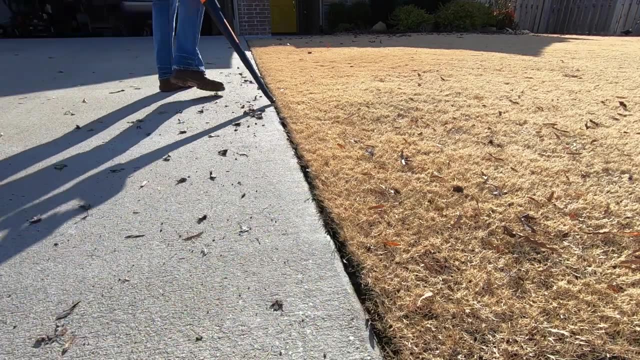 is a little matted down from the winter so far and Christmas lights are just up after the holidays, so I want to get out in the lawn and get whatever remaining leaves are left from the fall, out of the flower beds, out of the edges along the sidewalks and the driveway, and we're just 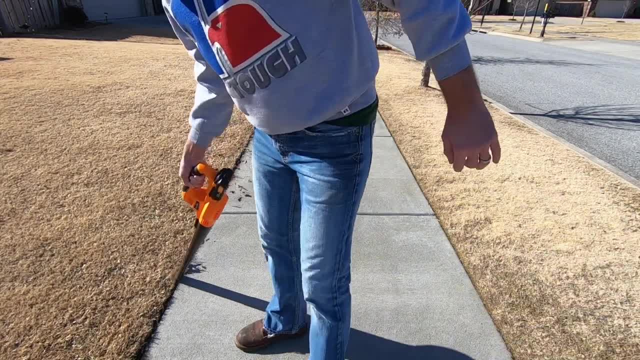 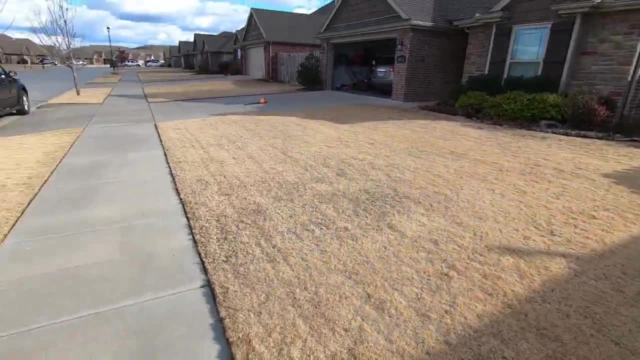 going to clean things up a little bit and fluff that grass up just to make it look a little bit prettier. Once we've got all the leaves up, we're going to run the lawnmower over it just a couple times to mulch things up, and that's pretty much it, And all this is doing is going to prepare us. 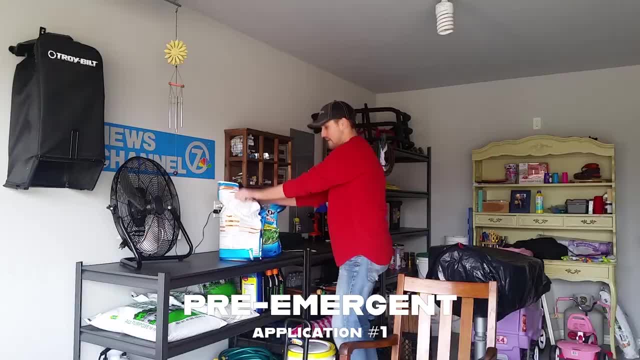 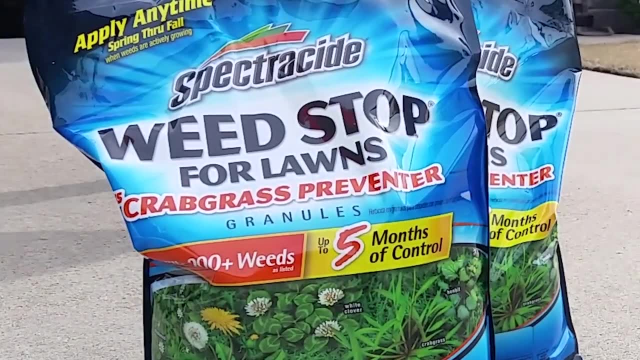 for our first major application of the year and that is a pre-emergent. We're going to time this to where maybe we have a little rain in the forecast, because this pre-emergent my favorite weed stop for lawns, plus crabgrass preventer. 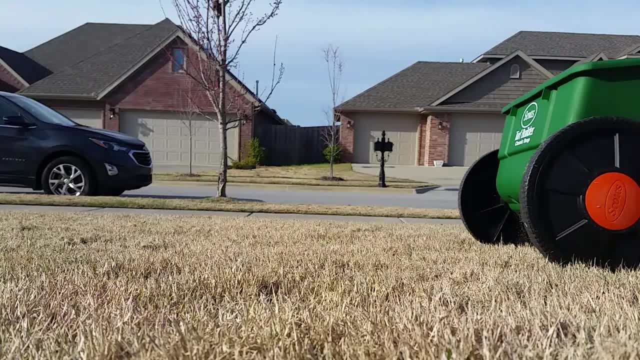 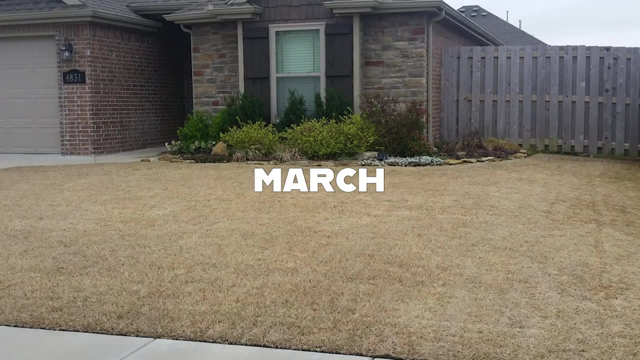 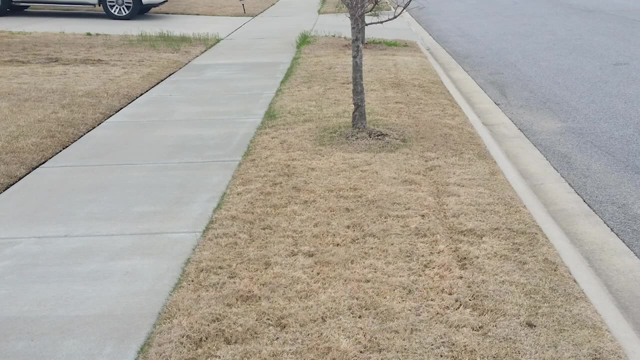 needs to be watered in to activate the ingredients. so we'll get that down sometime around the first of each year. Once that's on the ground, there's nothing left to do till March. Everything's looking good, no weeds in the lawn, but we've got to throw another round of that pre-emergent down. 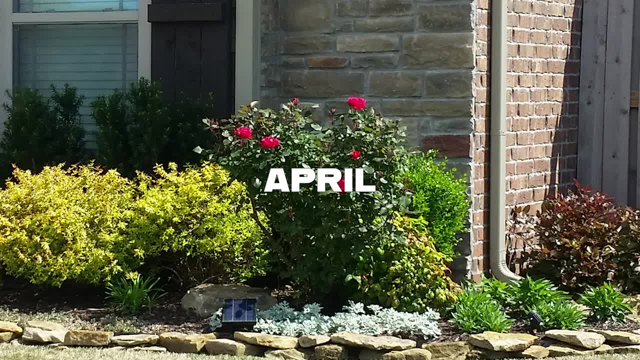 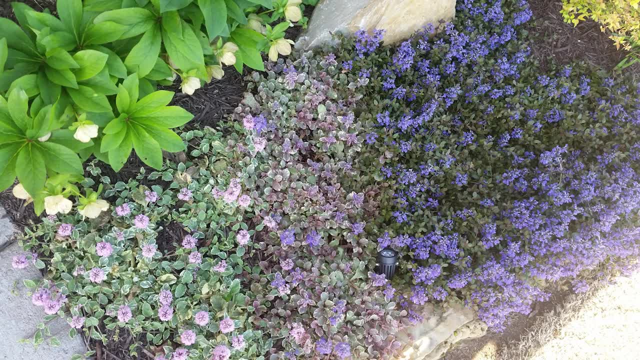 to prevent the crabgrass that could come up later in the spring and summer. Then we move into April. then we start getting into the swing of things. We're going to clean out our flower beds, get all the junk out of them, put new mulch down, pretty those up and then it's time to scalp. We need to. 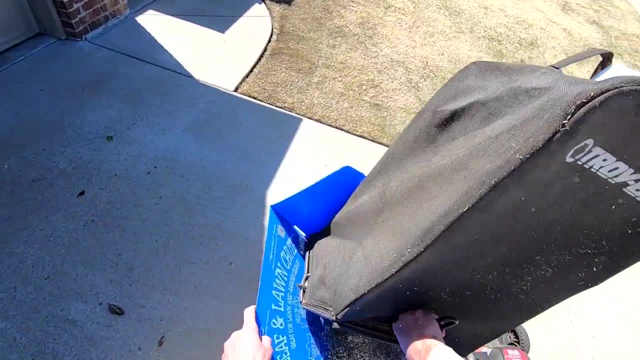 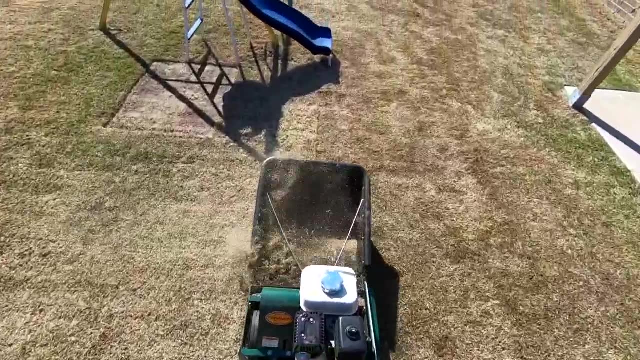 scalp that lawn down, open that turf and that soil up to some sunshine, some airflow and warmer temperatures, so we can start greening up a lot faster. I'll do it first with the rotary mower to get the worst of it up, and then we move on to the next step and that's going to be to get the 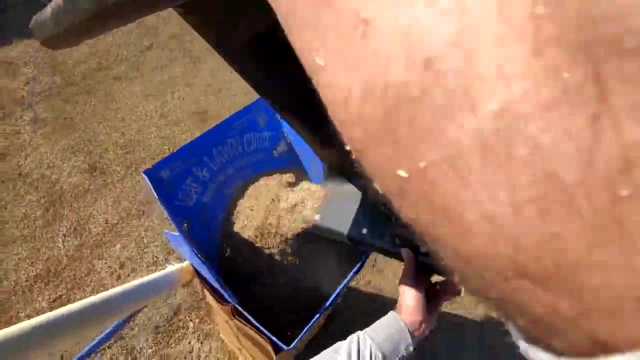 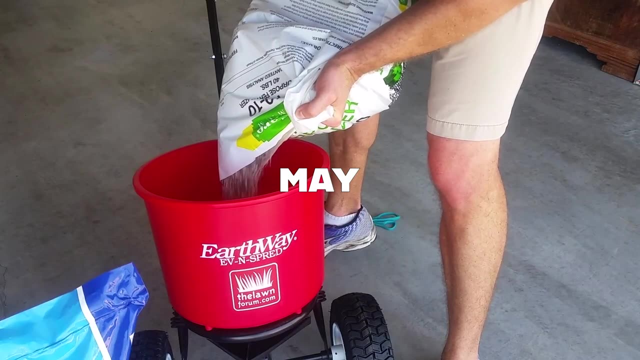 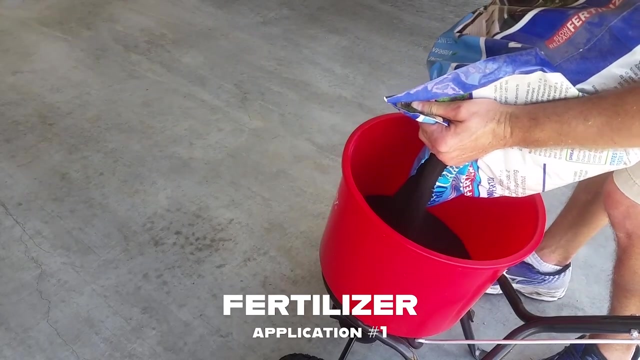 lawn over to the real mower to really get it down low, almost down to the dirt, and then we're going to start seeing things green up pretty quickly after that, Not going to do much for the rest of April until May. Then we start seeing our green grass really starting to show and it's time for 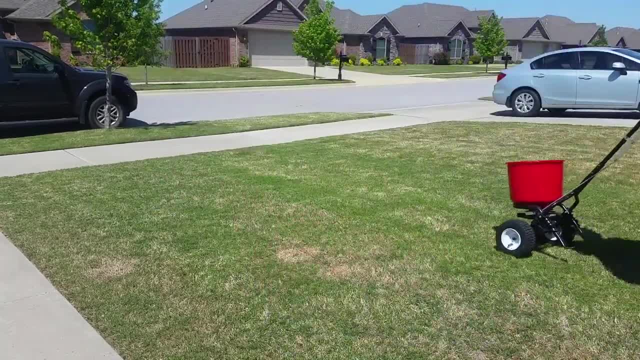 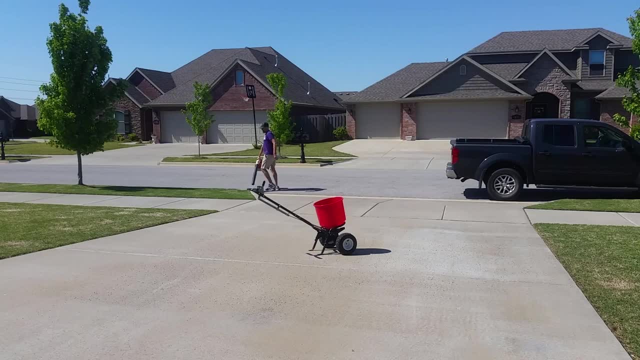 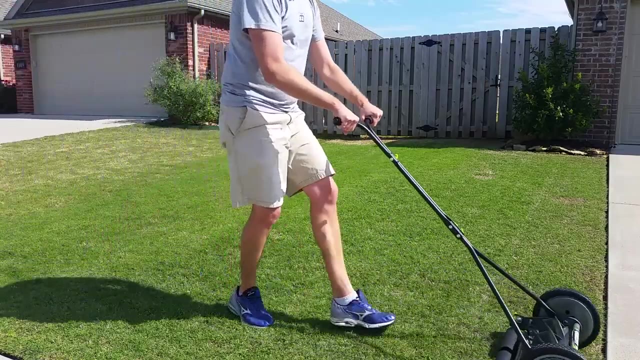 our first round of fertilizer. We're going to use a Triple 10 and just the ProCare Natural Organic, a little bit of both to get us both effects of a synthetic fertilizer and a slow-release organic fertilizer. That's going to be round number one in May and then from that. 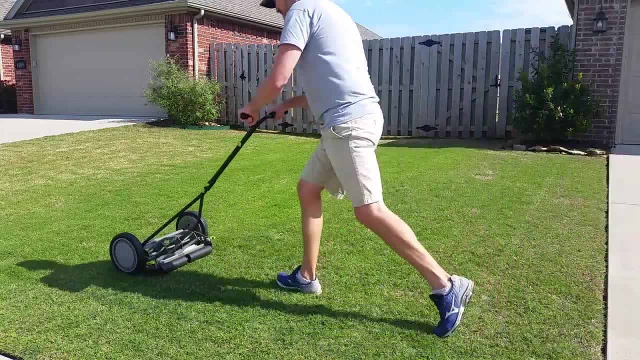 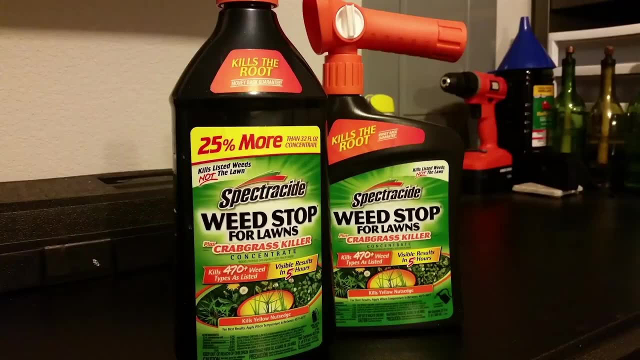 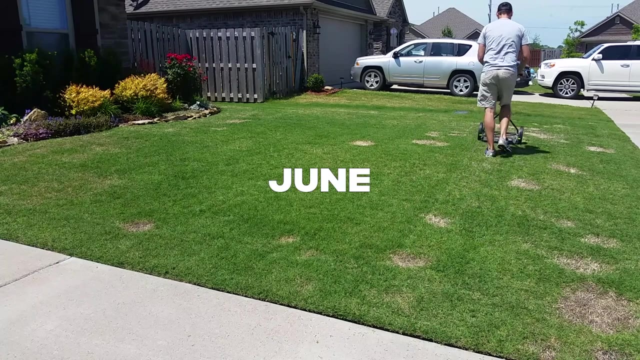 point on. it's just starting to get into our regular mowing routine. We're going to mow, probably not quite two to three times a week, but at least once a week at this point, and if we have any weeds popping up, that's when I like to use a post-emergent herbicide. in May Haven't had to deal with that. 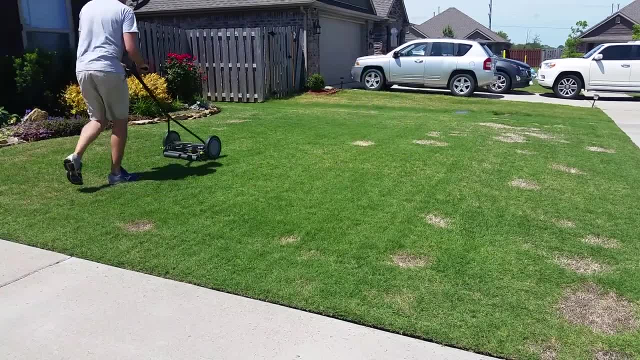 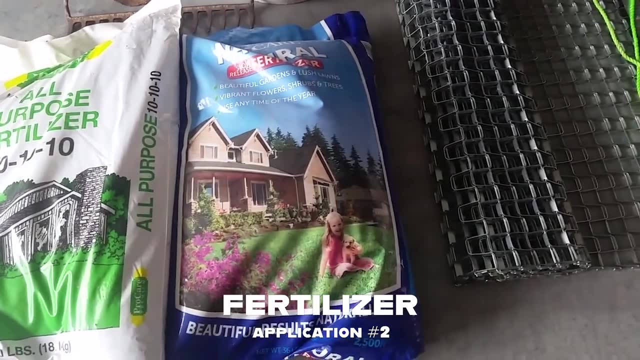 in some time, though. Here we are in June. Things are really starting to move now. You can see all pretty bad in my old lawn this time, but we're ready for our second application of fertilizer. We're going to time that around the time we want to level our lawn. I like to do the lawn leveling. 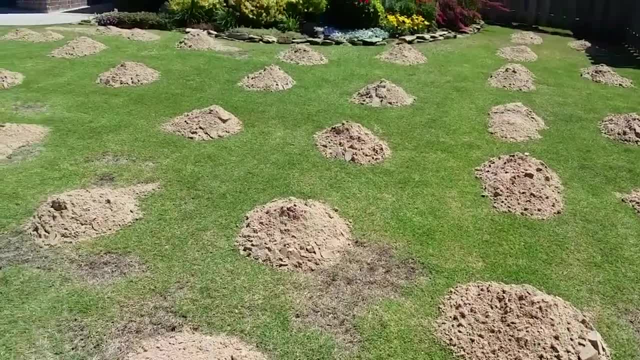 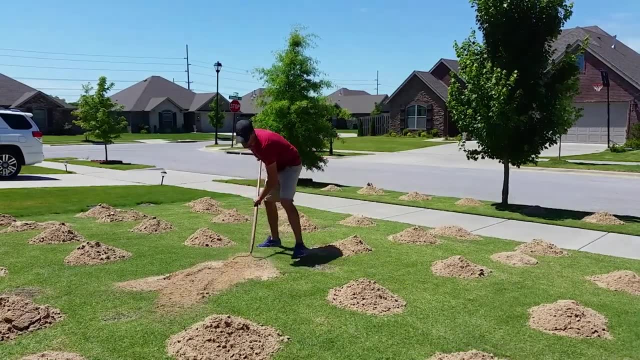 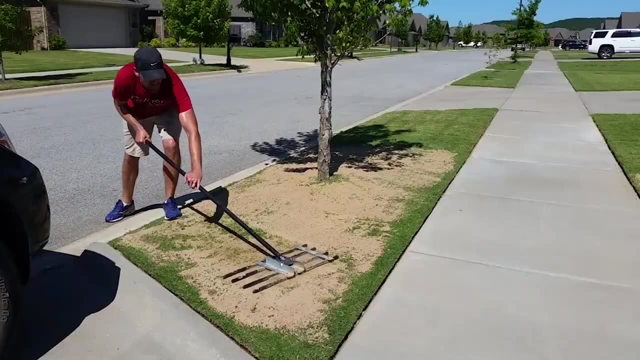 in June. That's when temperature's starting to warm up, The Bermuda grass starts actively growing. so, depending on your grass type, you want to make sure it's actively growing when you level your lawn. For me it's June. Some folks like to do it in July with Bermuda grass, but I want to. 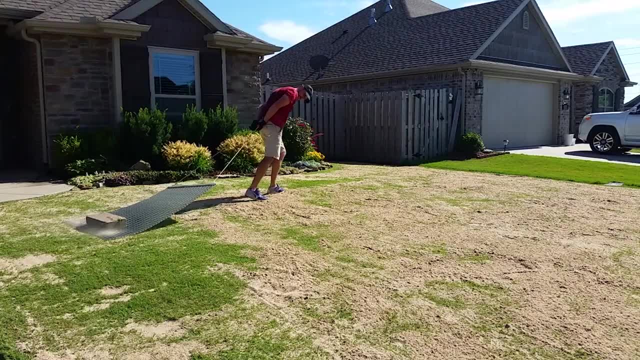 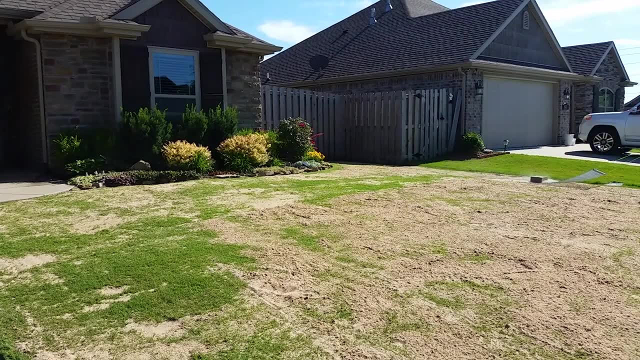 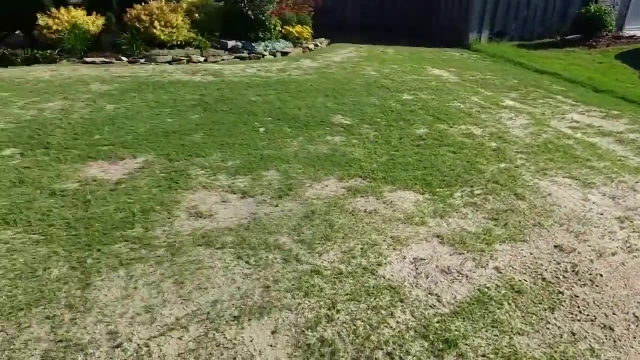 see the really bad heat. If you want to see how I do all these leveling projects. I've got videos about not only this, but everything else we're talking about in this video all across my channel, so go check out some of the other videos and you'll get more in-depth discussions about. 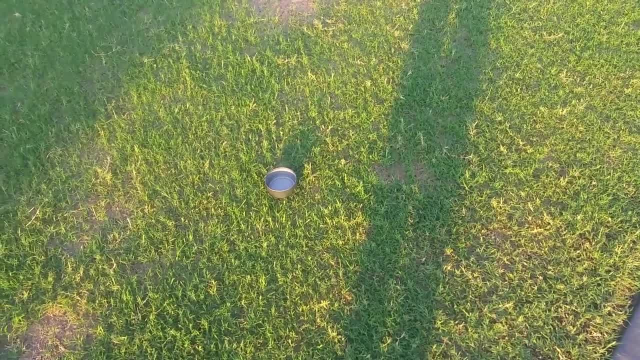 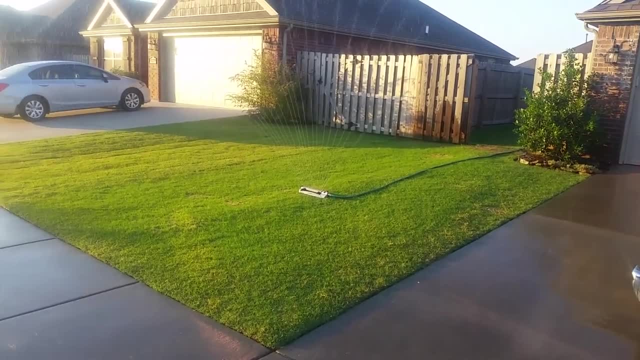 everything we're talking about here. Once we've got the leveling done, now we're just going to let that grass grow back in. We've got to make sure we keep it watered. At this point we're going to be on our pretty regular watering routine, trying to get around one inch a week. 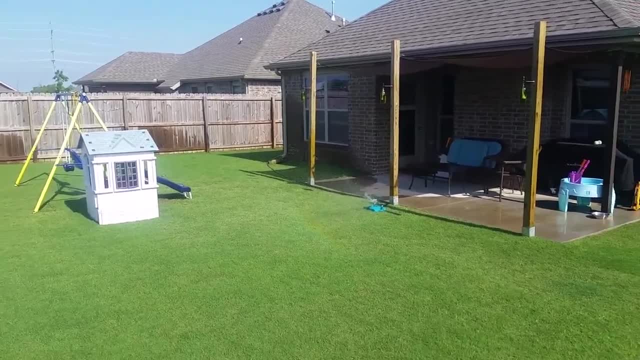 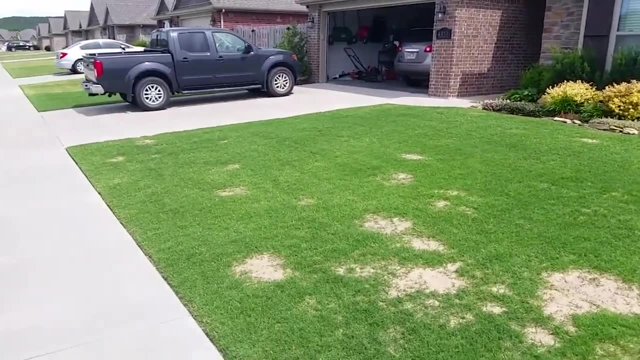 We're mowing a lot more at this time too, In June, especially heading into July, definitely mowing twice a week. but all that sand is starting to disappear. The more we mow, the more we water, the quicker it grows with those hotter temperatures. and then by the time 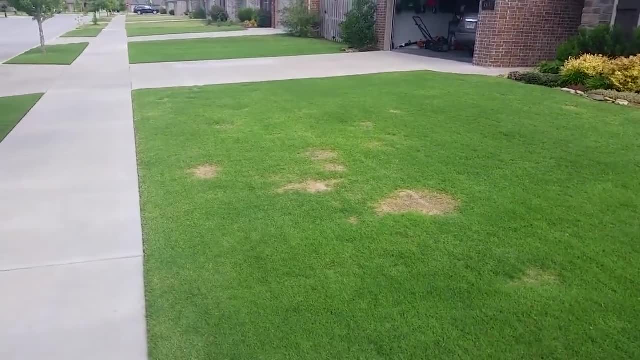 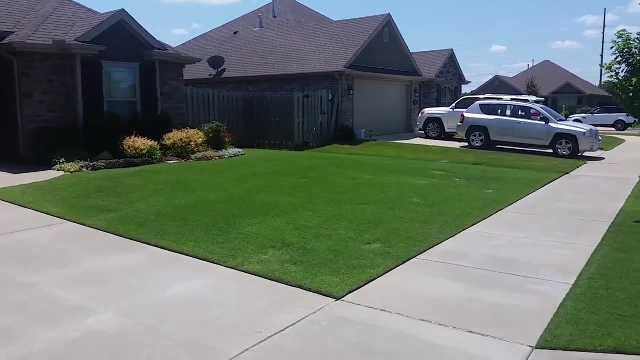 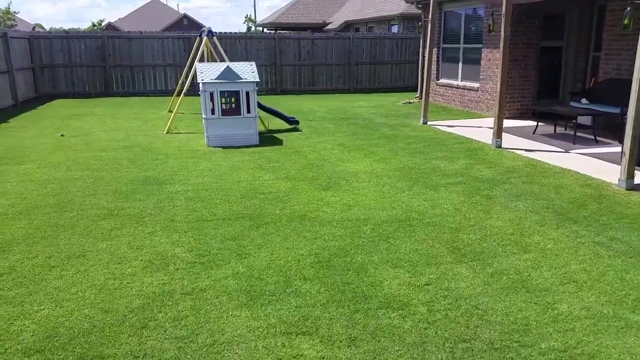 you know it. after covering your lawn with all that sand, guess what? You're back to normal, and it's so much better. at that point, Mowing is so much more enjoyable because you're not bouncing that lawnmower all over the place, and it's really starting to look good all across the lawn. Then 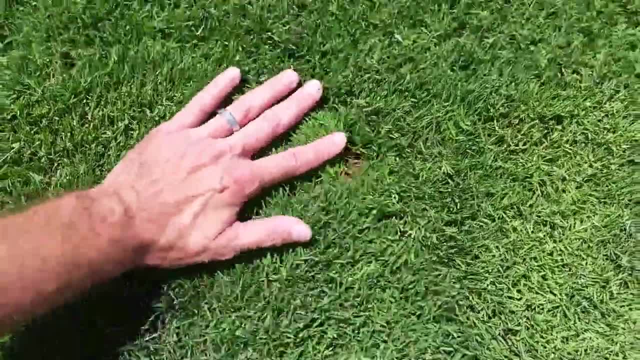 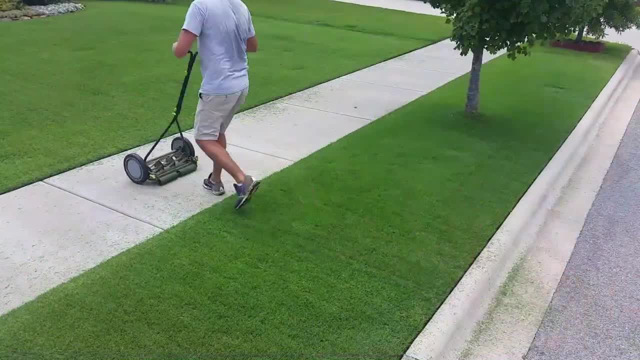 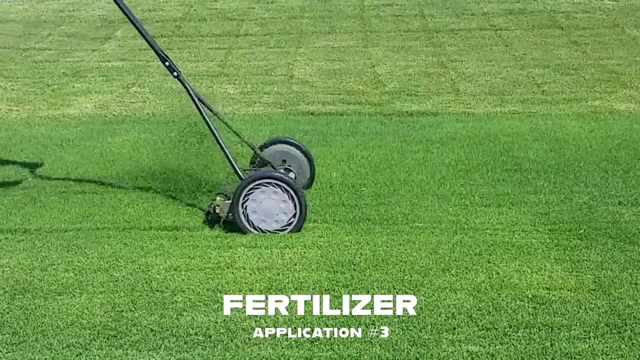 we're heading into the dog days of summer in July. Things are looking really, really good there, Just keeping up with our inch of water. a week, mowing, mowing and mowing some more. That's about all we really have to do in the really hot part of the summer. We're going to throw down our third round. 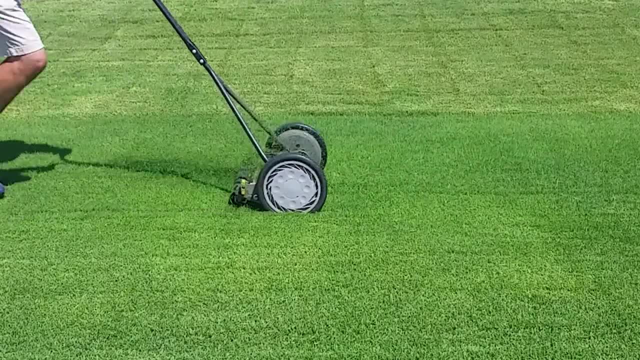 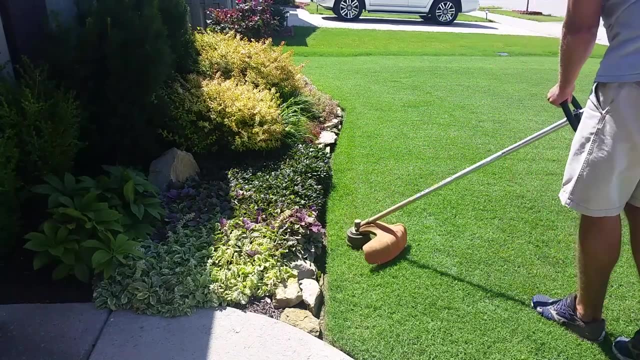 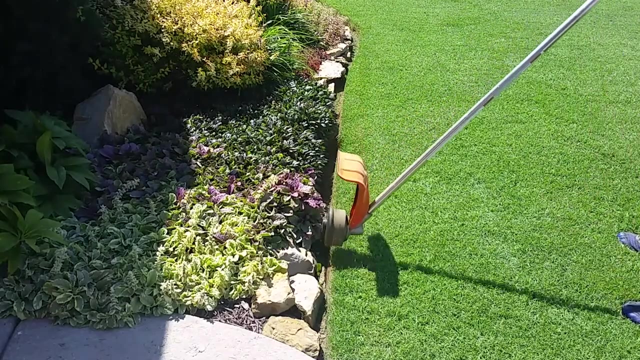 fertilizer in July as well, and just about the point where we start getting everything looking really in tip-top shape. The edges are looking awesome, The flower bed is looking sweet. We're just kind of in our normal routine of maintenance at this point. We've already done a lot of the 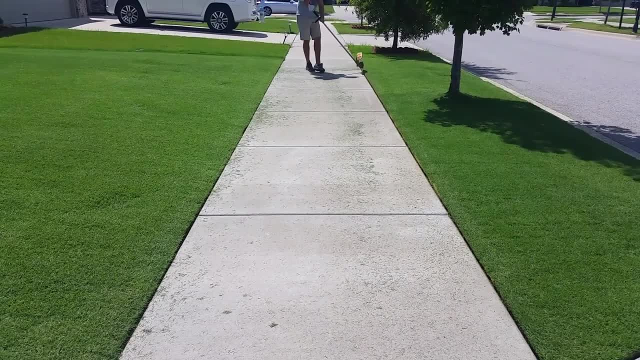 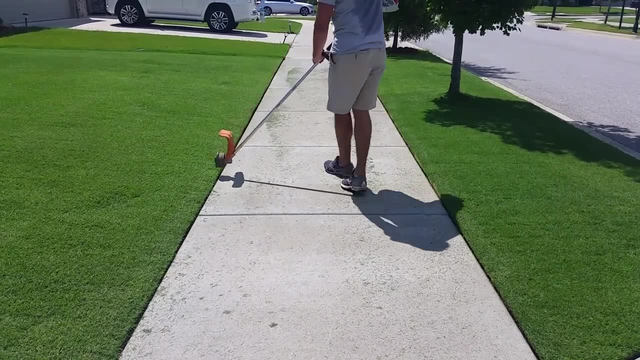 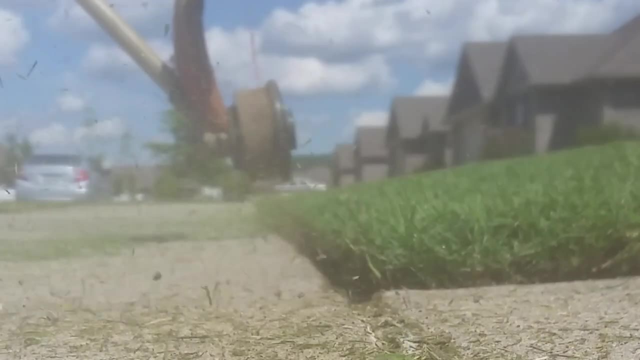 heavy lifting earlier in the spring. Things have kind of slowed down as far as major projects go. We're just doing our regular mowing, edging, blowing, watering and just trying to enjoy the summer. It's around 4th of July. Things are really cranking. 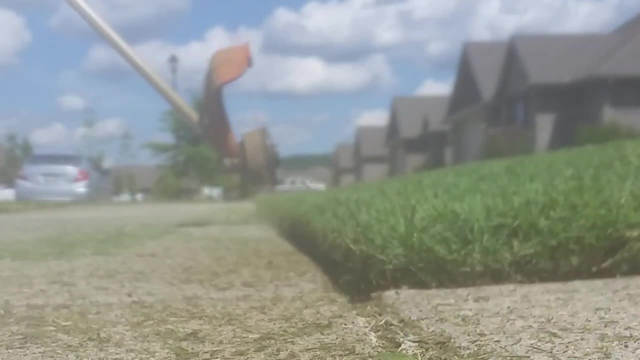 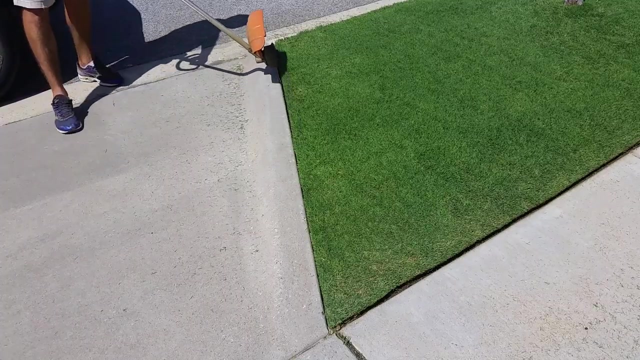 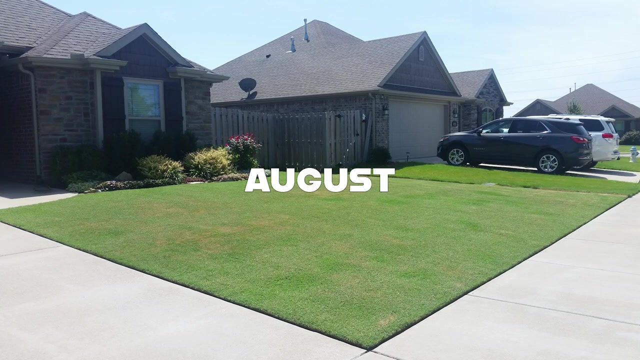 up with the summer activities. so we're taking it easy through most of the middle part of the summer. But I got bad news. If you get to this point and you think everything is just perfect, well, that brings us to another opportunity to mess it up as we head into August, and that's for our 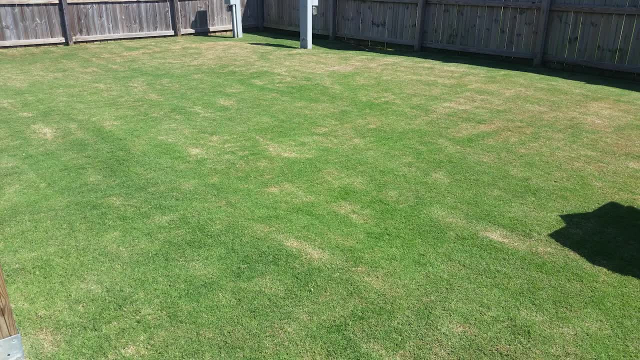 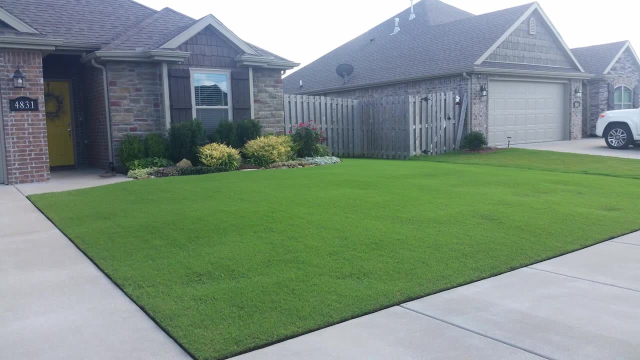 height of cut reset. We're going to scalp it down just a little bit more So we can reset things, but still give us time to grow back in through the end of August and into September. Here we are: in September time, The final application of fertilizer is going down. 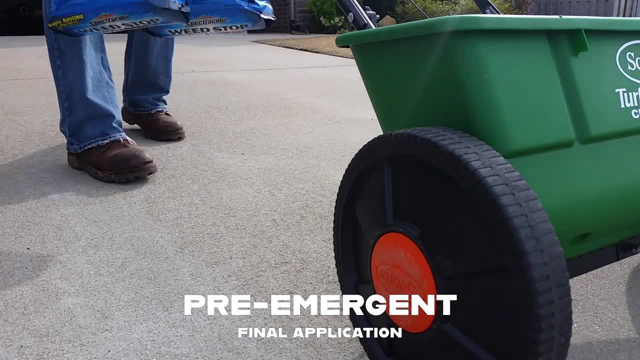 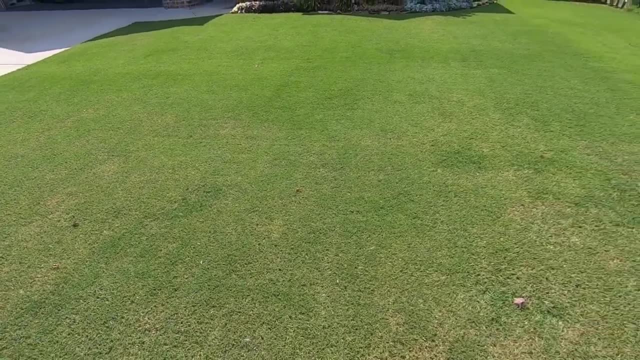 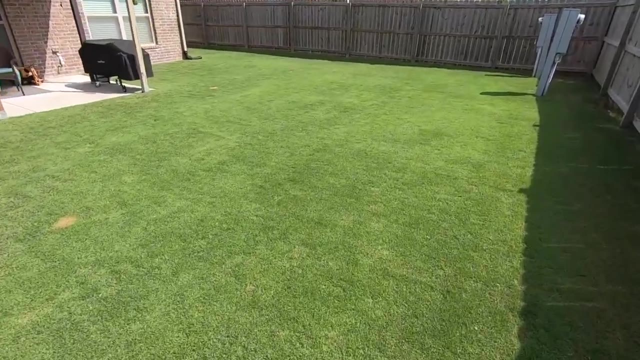 so is our final application of pre-emergent and we're getting this lawn ready to go back to sleep. Depending on your temperatures and location, in September, the days are getting shorter, temperatures are dropping, that color starts fading and we start seeing some of the first signs.